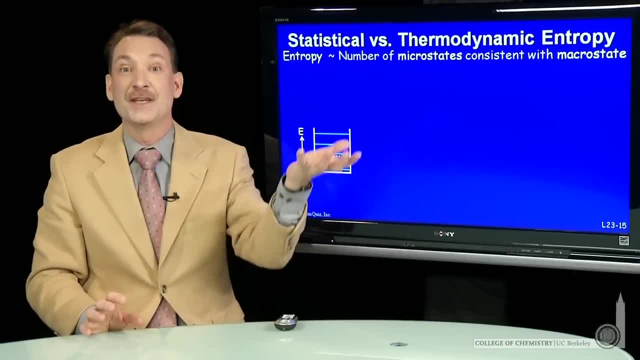 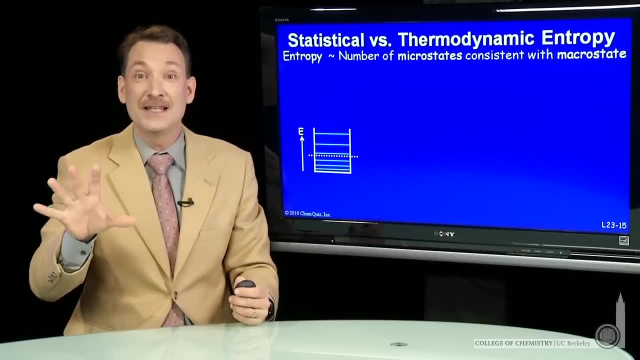 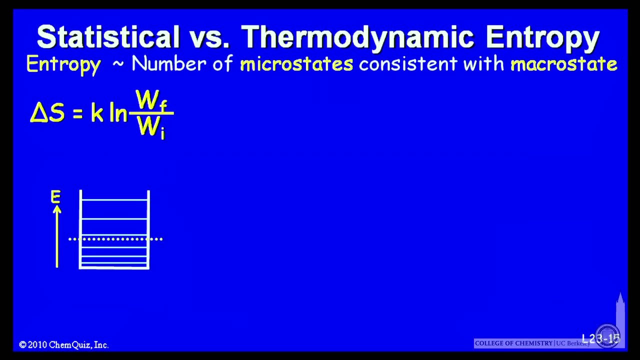 that says, as heat is transferred that entropy increases. So can I rationalize those two and bring them together as the same definition? Do they really mean the same thing? Well, it turns out they do. Here's the thermodynamic definition of change in entropy. the final number of microstates: 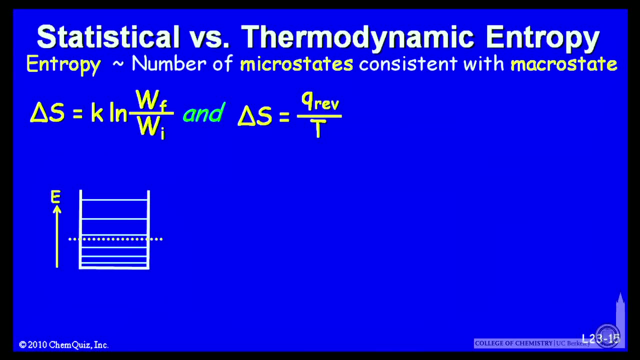 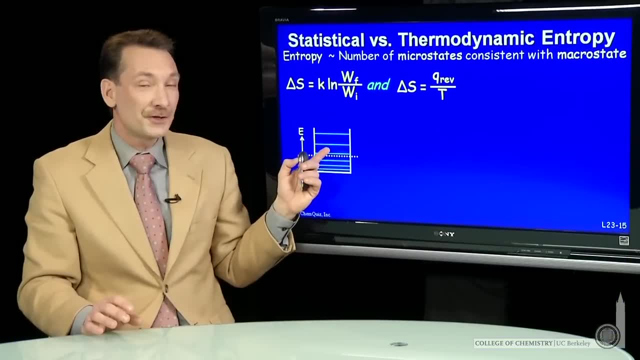 over the initial number of microstates, or the thermodynamic definition, the heat that a system absorbs at a specific temperature. Let's look at those both in terms of a system, say, like a particle in a box, a very simple system. 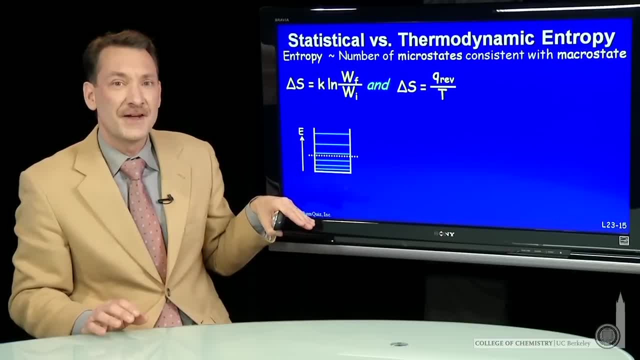 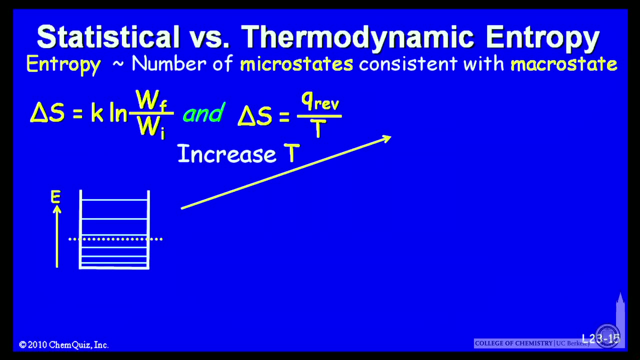 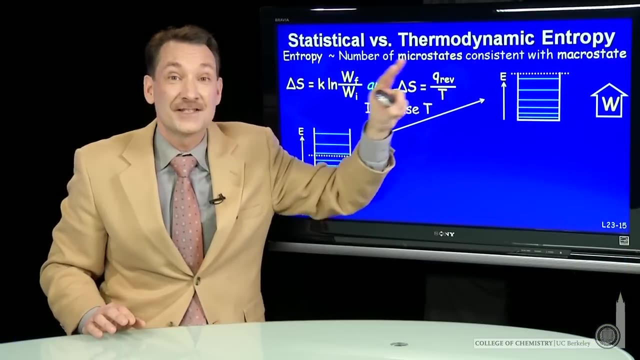 where there are several microstates available to the system. Now if you take that system and increase the temperature, that's increasing the energy. So I go from this energy state to this energy state. Now more microstates are available to the system. 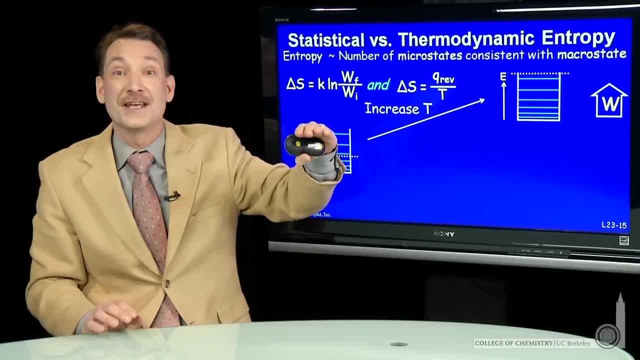 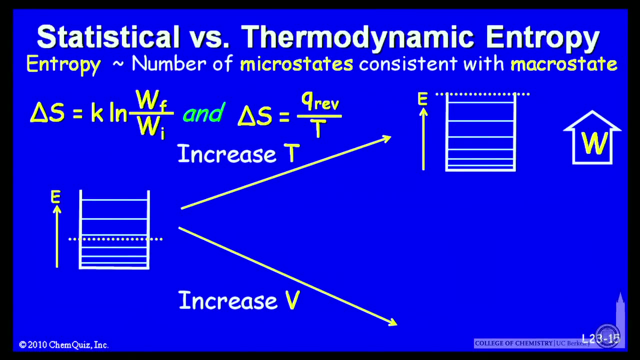 That is, I can distribute the energy over many more microstates. So that's an increase in the number of microstates. What if I increase the volume of the system? Well, you know, when you increase the volume of the system, as I increase the length of the particle, 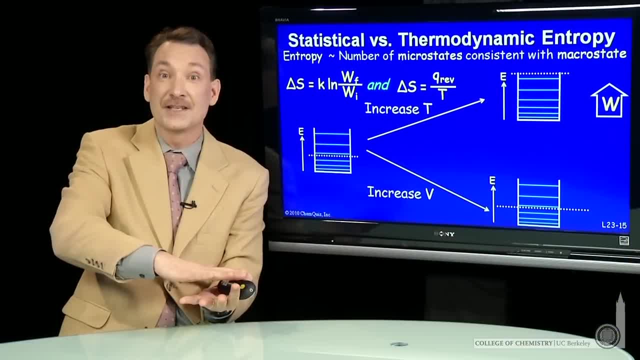 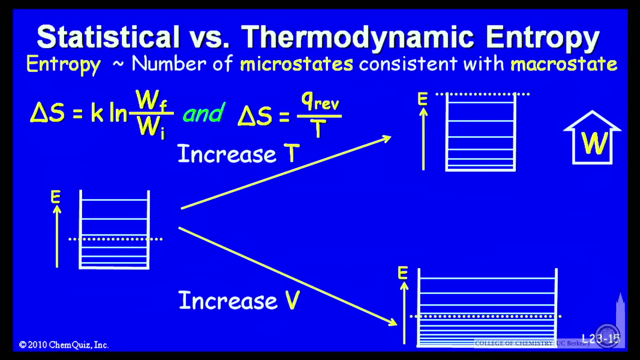 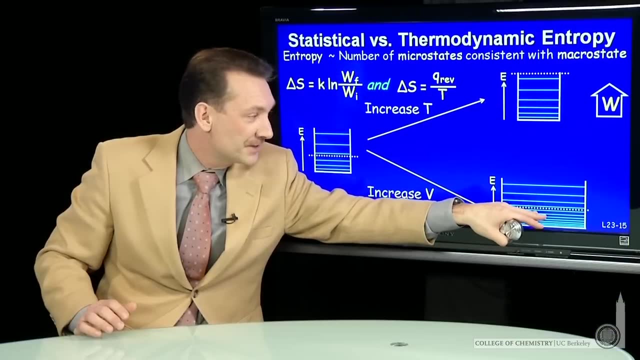 the energy levels collapse. They get lower in spacing. So increasing the volume decreases the spacing between my microstates. They get more compact And I get more microstates by increasing the volume as well. So more microstates accessible at this energy, more microstates accessible at this energy. 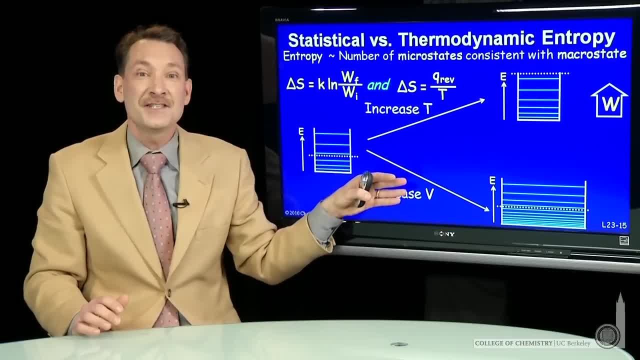 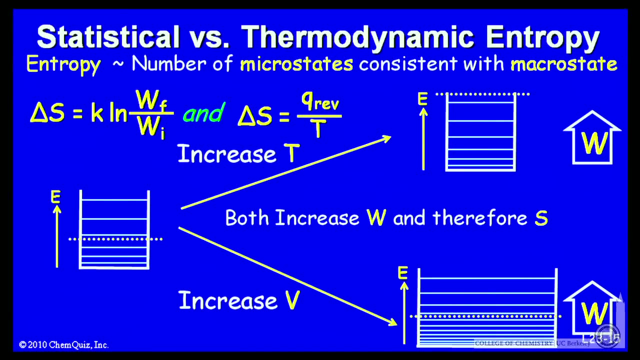 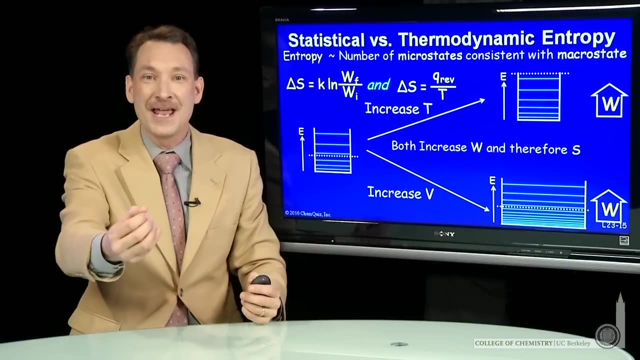 the temperature increase and the volume increase, a statistical and a thermodynamic definition of entropy. Both Increase the number of microstates, Both increase the number of microstates, Both increase entropy, And the thermodynamic and statistical definitions give us the same changes in entropy.